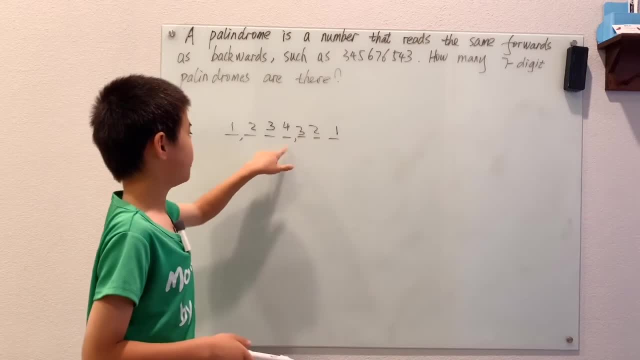 20,, 21, and 22, 21.. So that's the middle digit. Now, if you're reading it backwards, well, 1, 2, 3, 4, 3, 2, 1.. It's the same number. 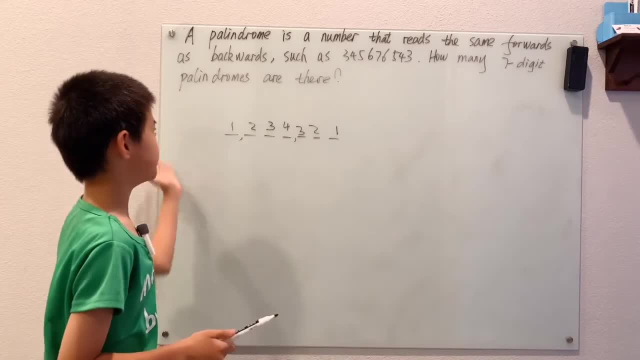 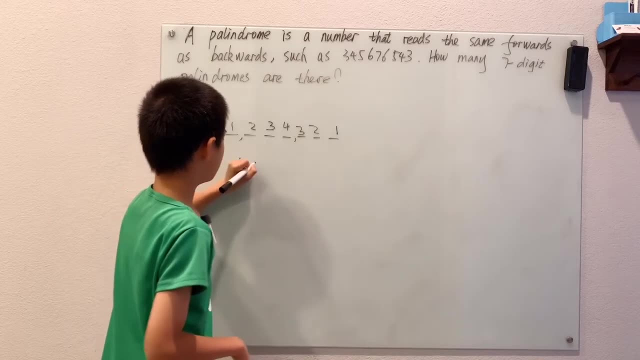 forwards and backwards. So now we kind of get an idea of how these 7-digit palindromes are formed. So basically you just have some kind of 3 numbers at the beginning- a, b, c, some 3-digit number- And then after that there's the middle digit, x. that doesn't. 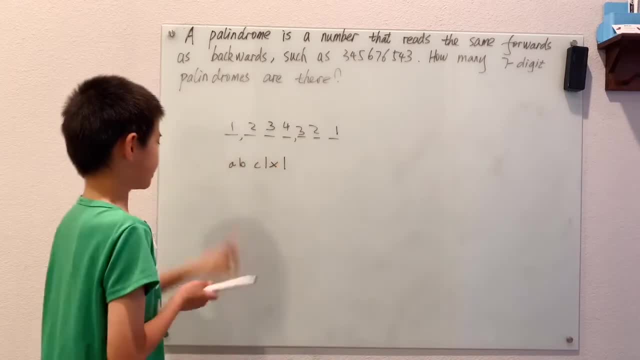 really change at all, And then after that it's just a, b, c, only it's a b, c. 4, 3, 2, 3, 4, 5, 6, 7, 8,, 9, 10,, 12,, 21,, 13,, 18,, 19,, 20, 21,, 22,, 23,, 24,, 24,, 25,, 26,, 27,, 28,, 28,, 29,. 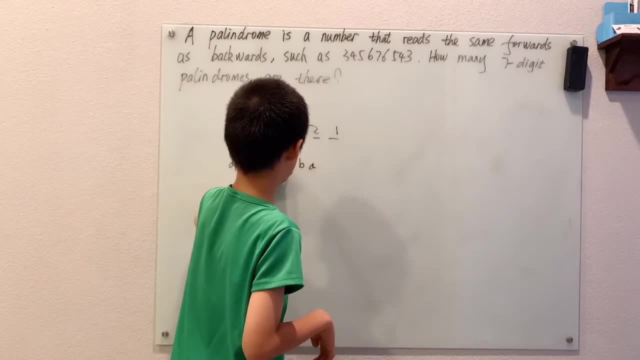 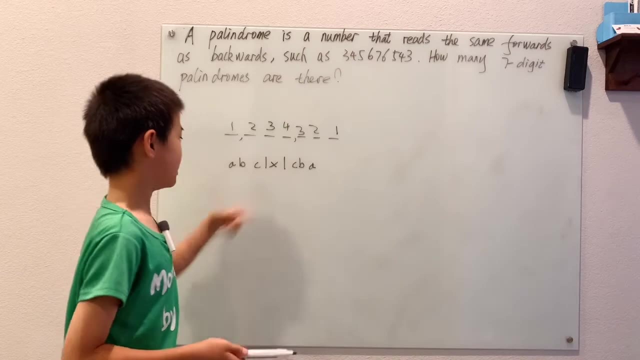 from the back. So A, B, C, And you can say, well, A, B, C, X C, B A, A B C, X, C, B A, So it's the same thing forwards and backwards. So basically, just how many ways can you do this? 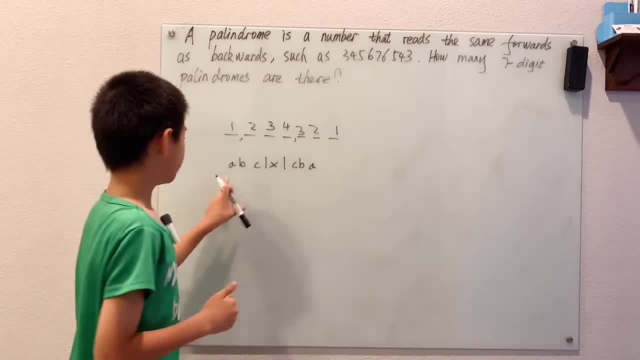 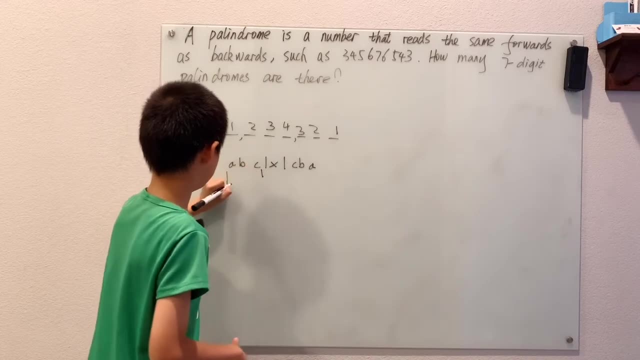 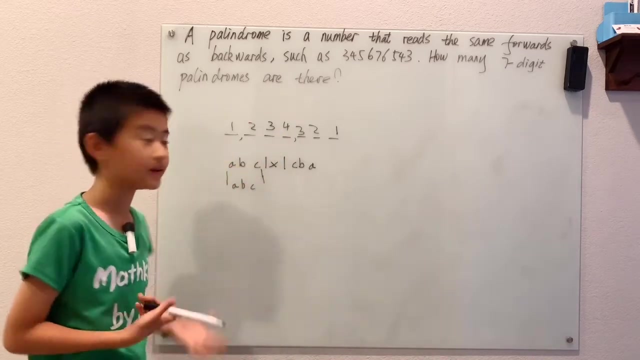 Now it looks complicated, but it really isn't if you think about it. So, first of all, number of addition numbers. I'll figure that out later, So I'll just put that in here: A, B, C. Well then for X. well, X is just a single digit, right Four. It can't be 600. since you can't 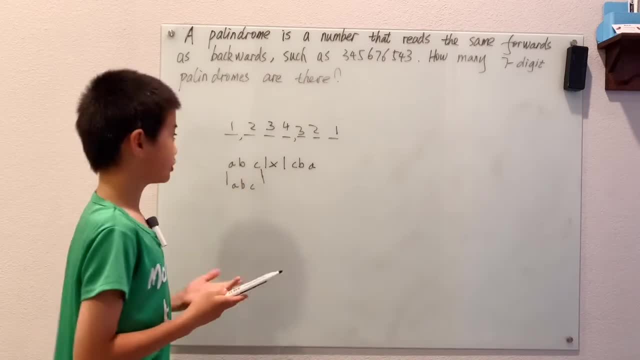 well then it's not a digit, So for X. and then there's just well, first of all it can be zero, right, Since it's not at the beginning and there's no restrictions, that it can't be zero. 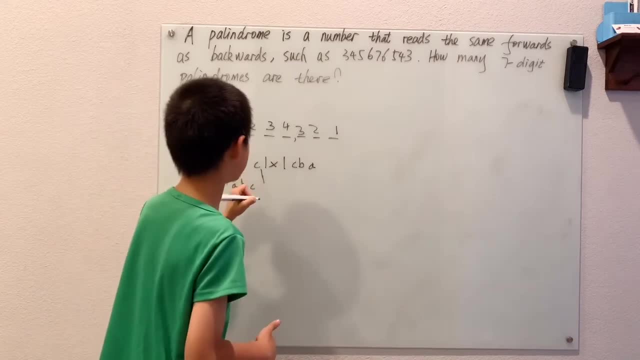 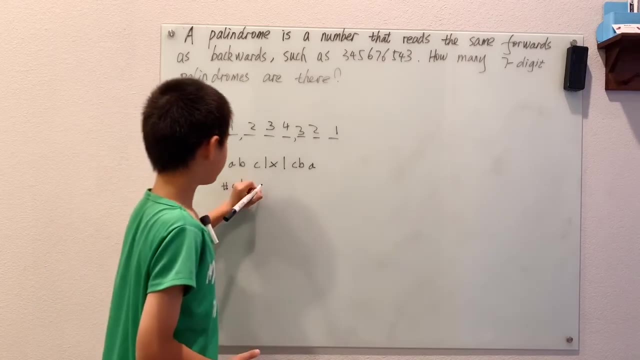 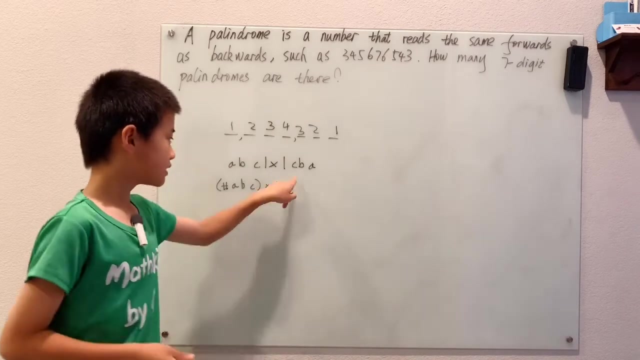 So it has zero, one, two, three, four, five, six, seven, eight and nine, which means really it's just number of ways to do A, B, C times, while the number of possibilities for X is just 10.. Now the C, B, A, if you think about it. 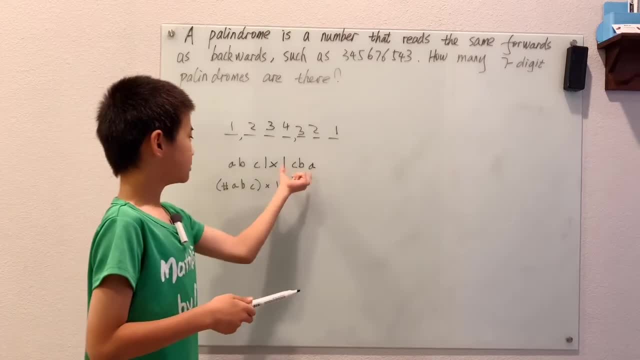 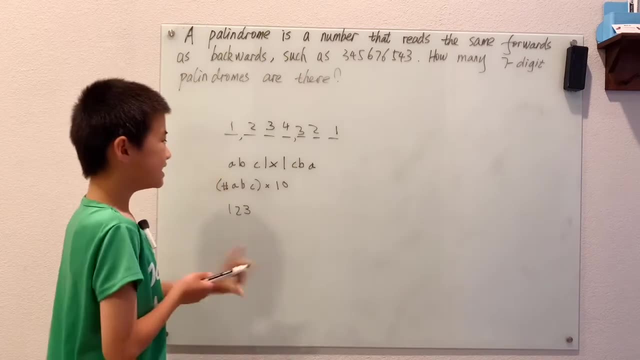 we don't need to do that. In fact we can't do that because, well, C, B, A is just A, B, C, like swap, right? So if A, B, C is one, two, three, as we see up here, C, B doesn't have a. 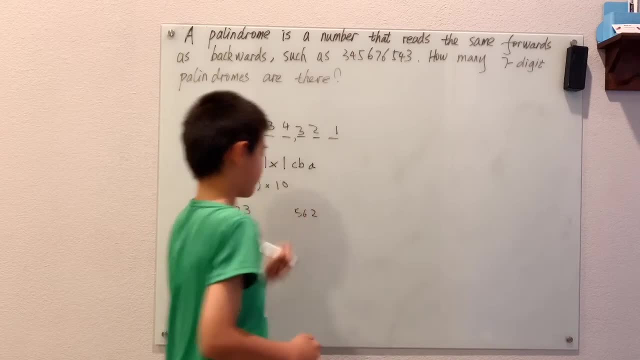 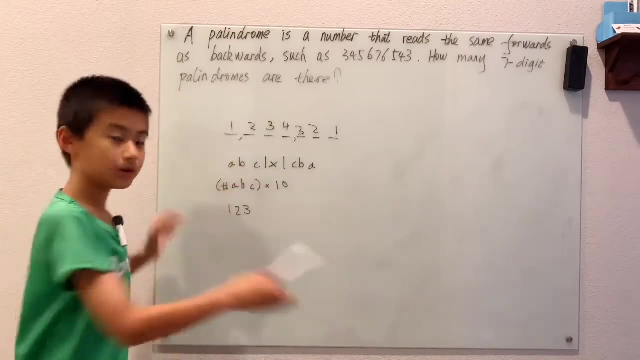 choice right Like C, B, A can't be like five, six, two, since that isn't the backwards of one, two, three, meaning whatever A, B, C is, C, B A has to be the opposite of that.